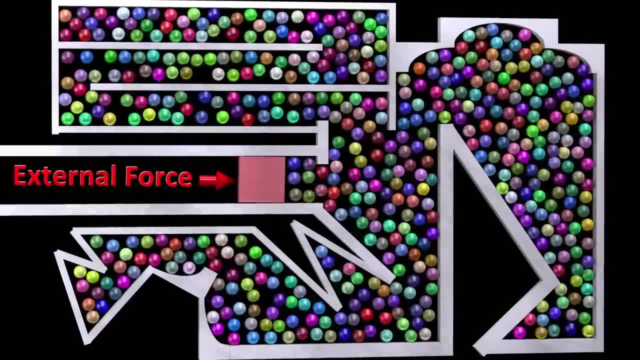 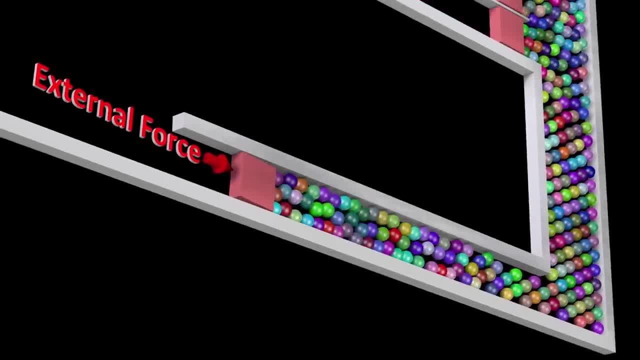 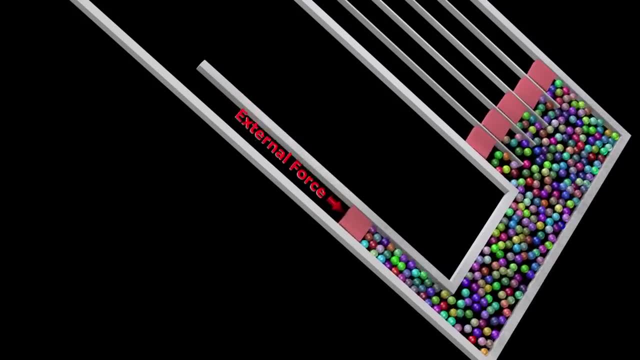 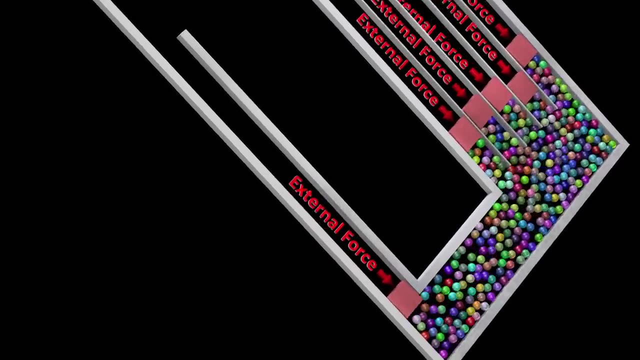 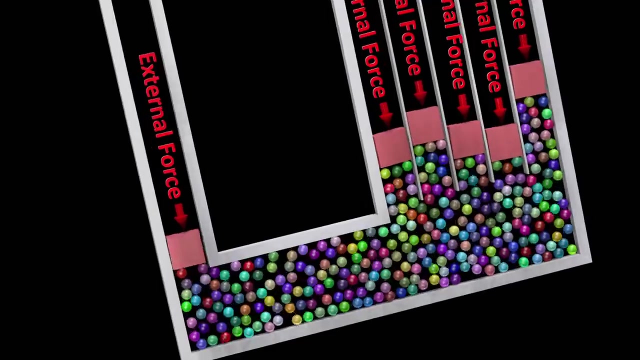 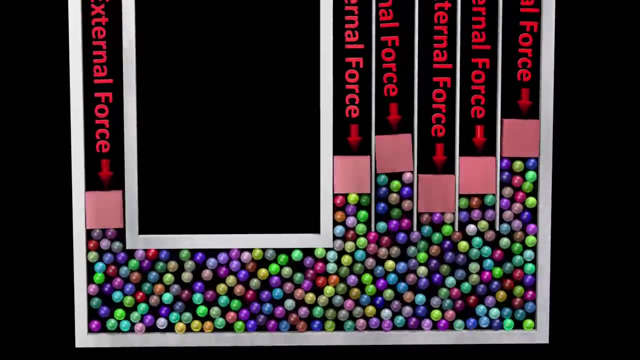 Let us now consider a slightly different scenario. Let us also apply an equal external force on each of the other red rectangles, Since the pressure of the fluid is the same everywhere. this pressure balances each of these external forces. As before, we are in a zero-gravity environment. 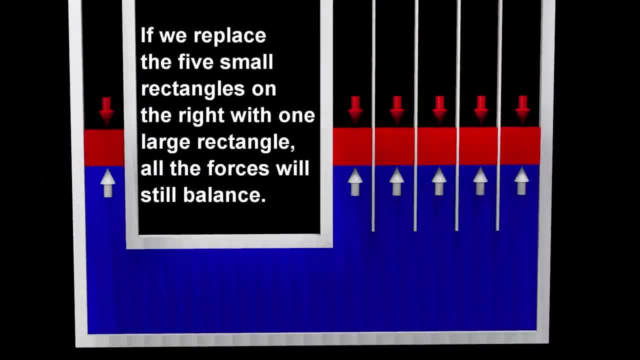 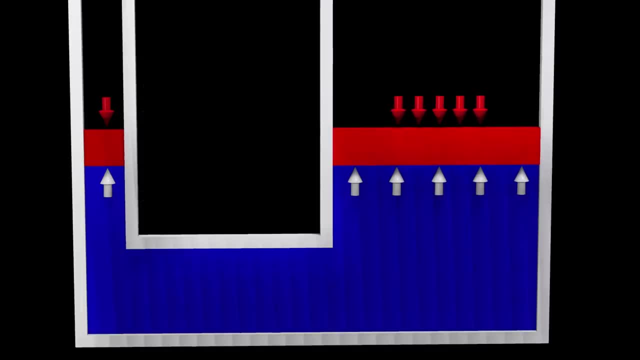 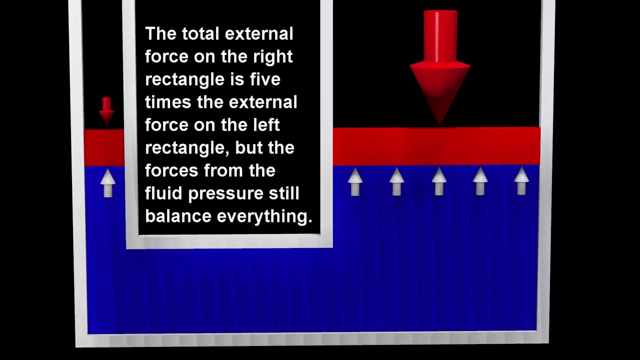 If we replace the five small rectangles on the right with one large rectangle, all the forces will still balance. The total external force on the right rectangle is five times the external force on the left rectangle, But the forces from the fluid pressure still balance. 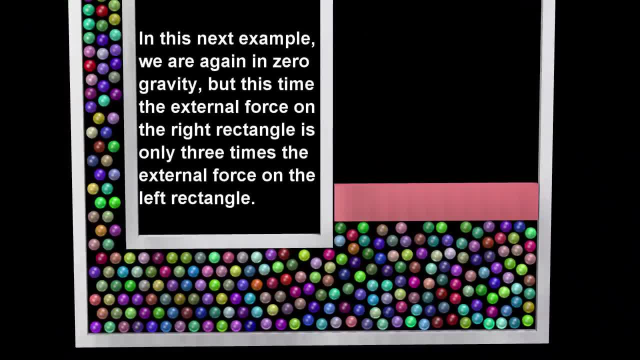 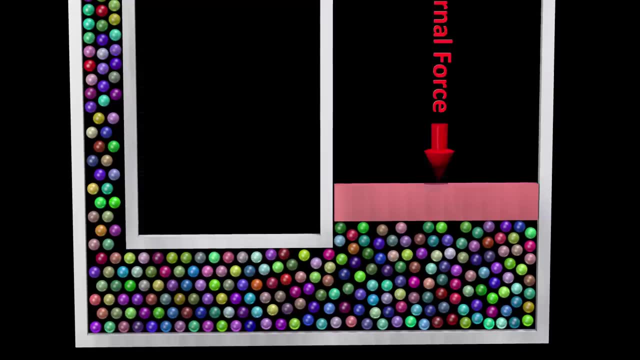 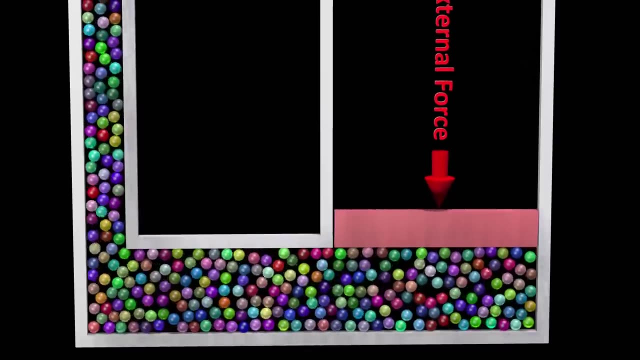 In this next example we are again in zero-gravity, But this time the external force on the right rectangle is only three times the external force on the left rectangle. If we replace the external force on the left rectangle with the external force on the right rectangle, the total external force on the right rectangle is three times the external force on the right rectangle. 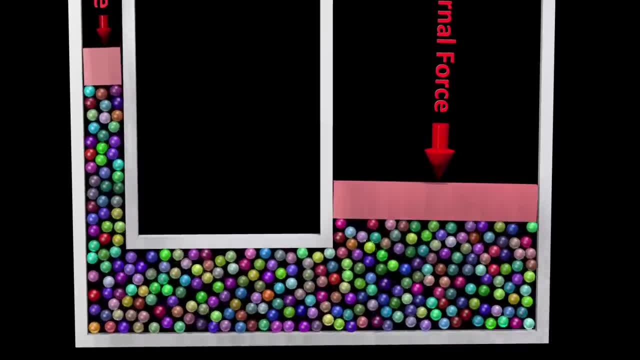 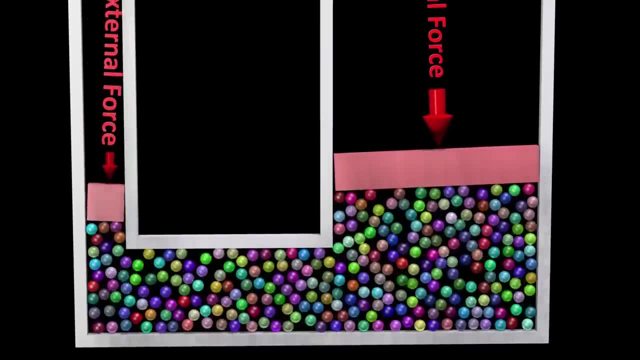 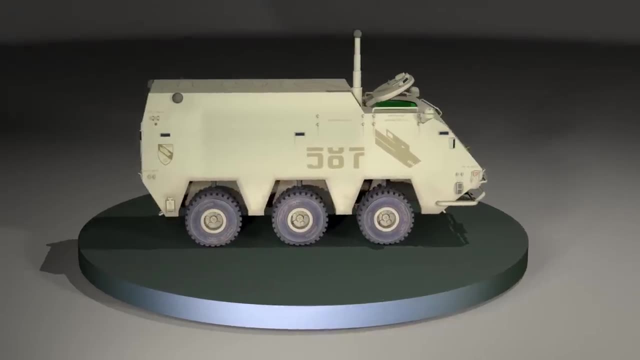 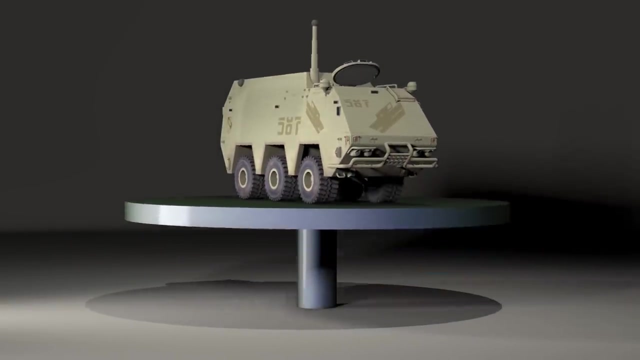 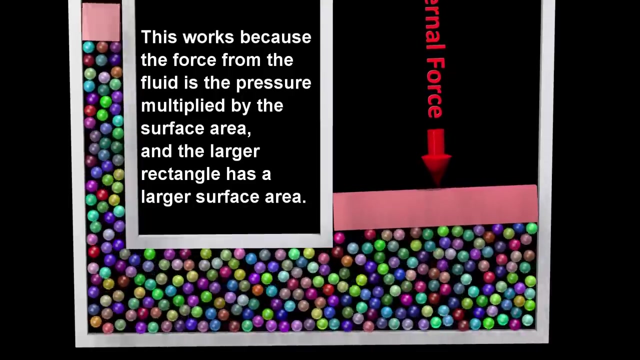 Here the smaller force manages to overcome the larger force. There are many practical applications of this principle, such as the hydraulic lift, which allows us to raise extremely heavy objects. This works because the force from the fluid is the pressure multiplied by the surface. 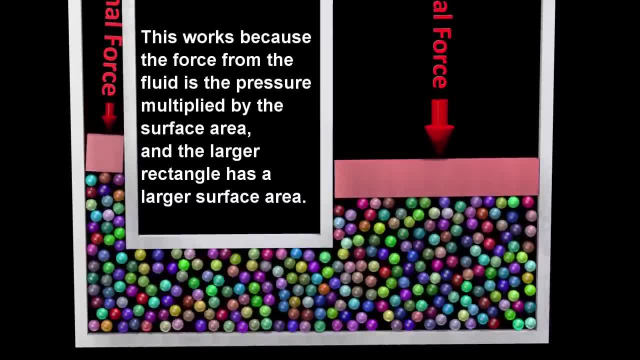 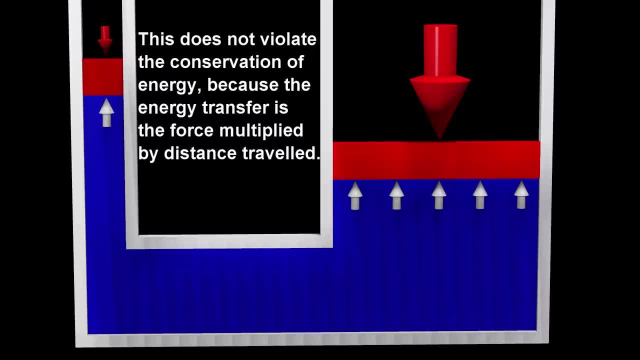 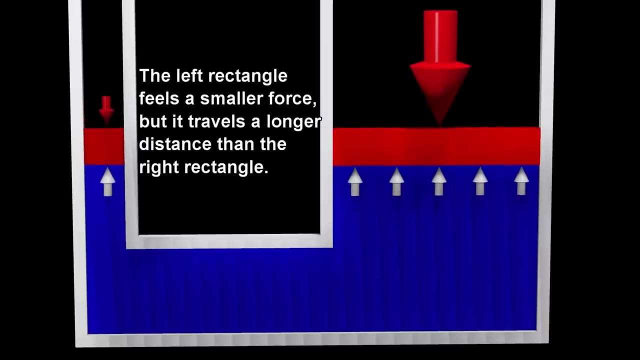 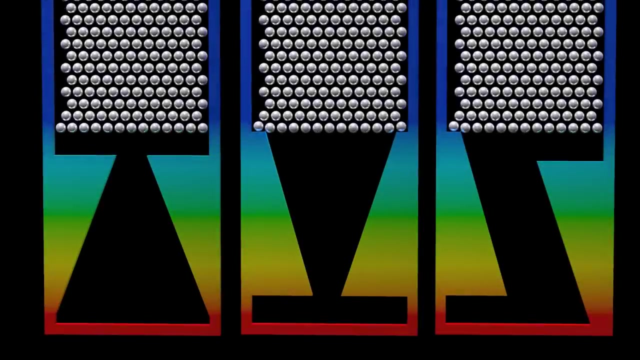 area and the larger rectangle has a larger surface area. This does not violate the conservation of energy, because the energy transfer is the force multiplied by distance traveled. The left rectangle feels a smaller force, But it travels a longer distance than the right rectangle.